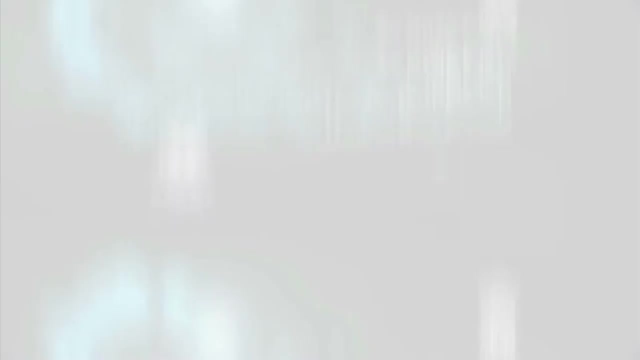 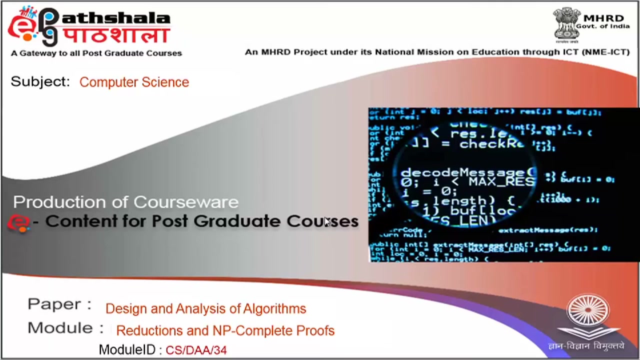 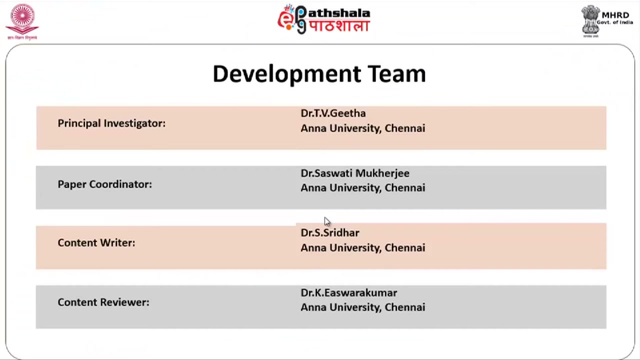 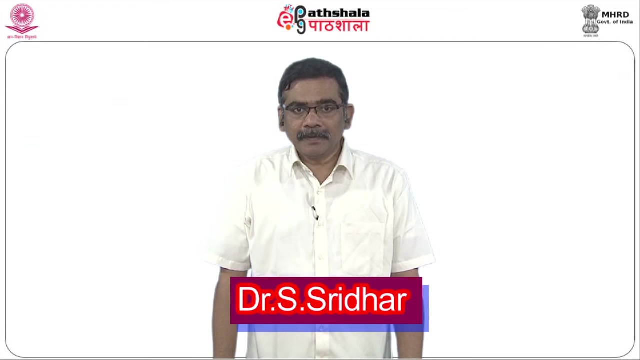 Welcome to E Podasala lecture series in computer science. In this module we are going to discuss about the proof of NP complete problems. Last module we discussed about some of the fundamentals of NP complete problems and at the end of the module I gave a simple example of how. 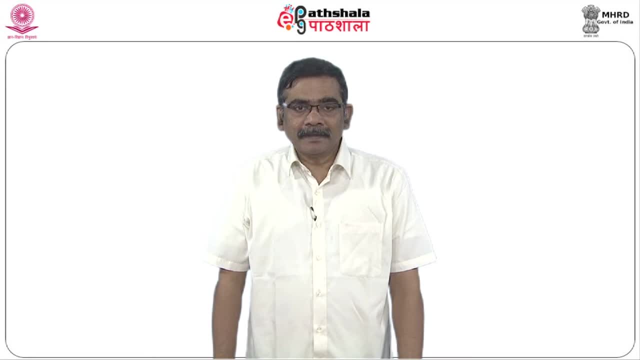 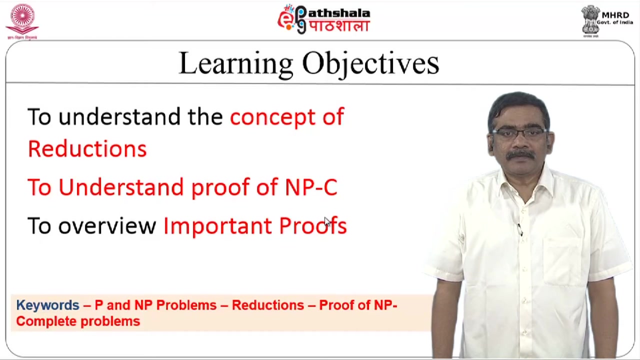 the NP complete problem can be characterized. In this particular module, we will discuss about how to give proof for NP completeness. In this module, we are going to discuss about the concept of reductions, which is one of the most important fundamental of NP complete. 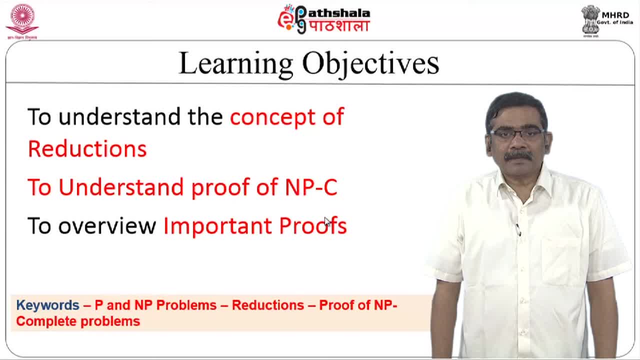 problems. We will talk about Karp reduction, which is useful for giving proof of NP completeness. We will also discuss about some of the proofing techniques. We will try to understand how the proofs are given for NP complete problems And we will also overview some of the important proofs of NPC. First we will start the discussion. 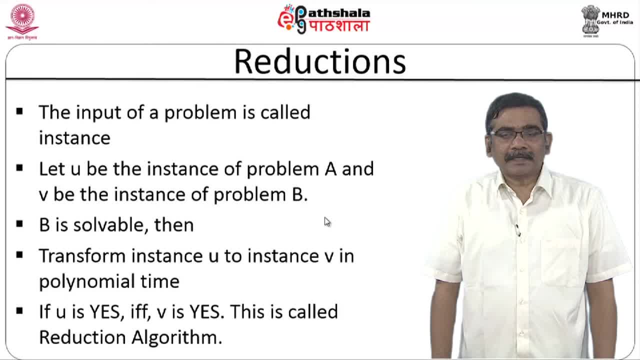 of reductions. What is a reduction? Reduction is we can reduce a problem to another problem. This is called problem reduction strategy. Probably you can recollect, in the module titled transform and conquer, we had seen that some problems can be converted to another. 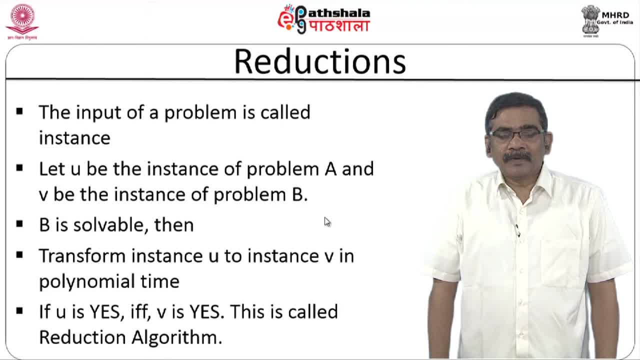 domain where things are very easy, where we can solve those problems and the results can be mapped to the original domain. For example, if I want to multiply two numbers in Arabic, then I may not feel very comfortable with that, So I may convert that to some other number. I can do some sort of an operation and I can. 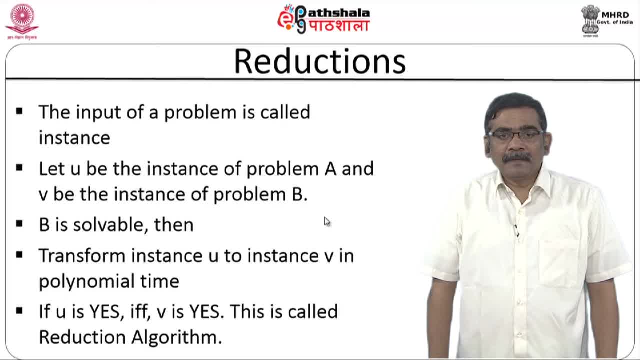 do the result back. Similarly, if I am not very much comfortable with Roman system, then I can convert the Roman numbers to Arabic numbers where the manipulation can be carried out and the result can be mapped to the original domain. Suppose if the input of a problem is called an instance. let us assume that two problems 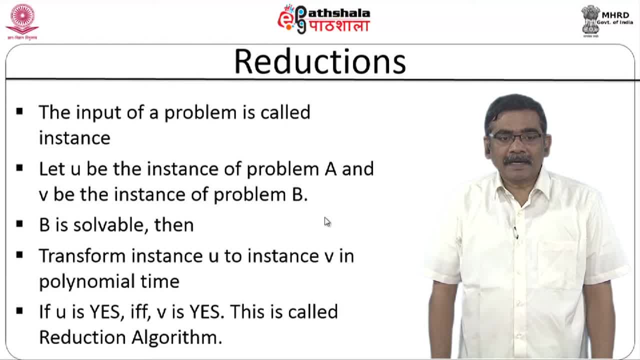 are available: problem A and problem B. u is the instance of problem A and v is the instance of problem B. Let us assume that we have a solution for B, but we do not have the solution for problem A. If that is the case, then what we can do is we can transform. 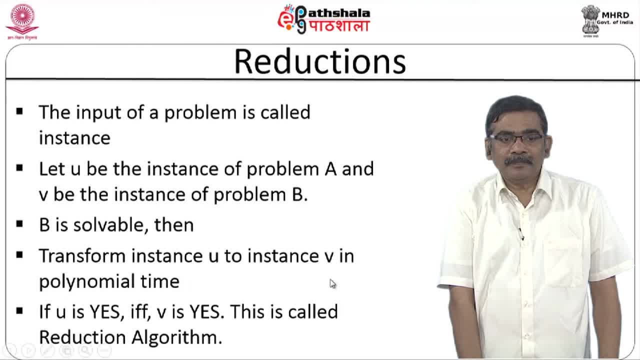 the instance U to instance V in polynomial time and we can use the solution of the problem B as a subroutine to solve that and we can say that the solution is the solution of the original problem A if U is F, S and simultaneously V is also S, In other words, if the 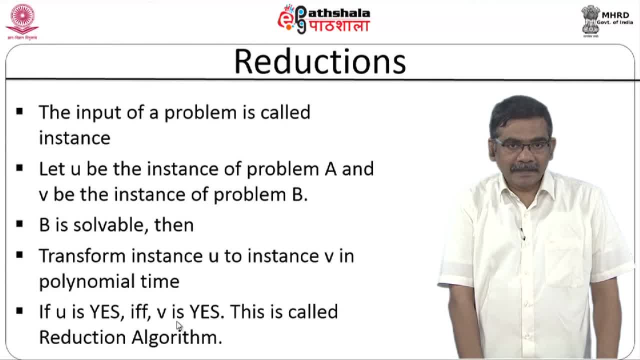 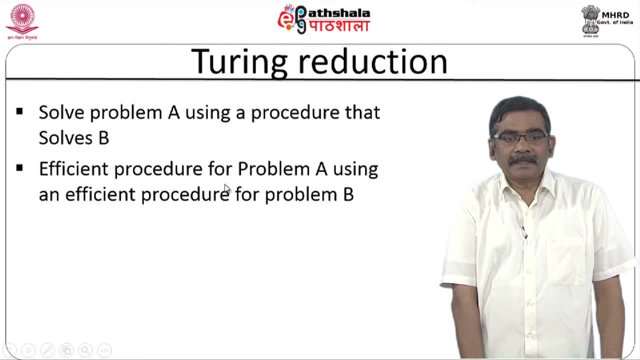 instances are equivalent, then we can say that the solutions are also equivalent. So this kind of strategy is what we are calling as the reduction strategy. In other words, Turing reduction is solving a problem A using a procedure that solves the problem B. In other words, we can use that solver as a subroutine to solve the given. 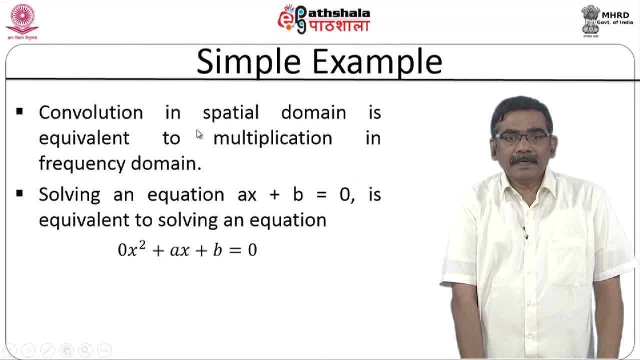 problem A. We can take a simple example as part of problem reduction strategy, Convolution in spatial domain is equivalent to multiplication in frequency domain. Say, for example, if I want to convolt two signals, the same problem can be solved by transforming that spatial data to frequency domain data, where we can do applying multiplication and 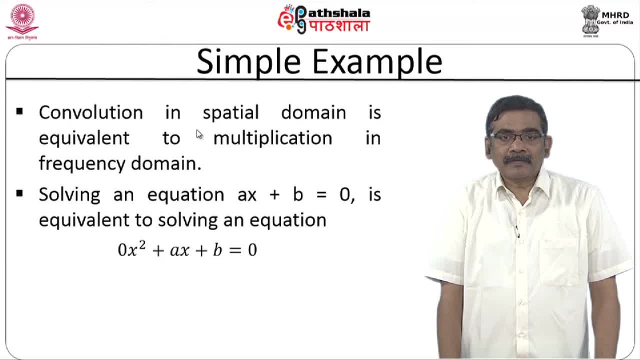 we can apply the inverse information of the gravity. One is suppose dos and aqui has FFT to get back the original data, which is a solution of the convolution problem. Simplistically, if I want to solve a problem A X plus B, then this problem can be transformed. 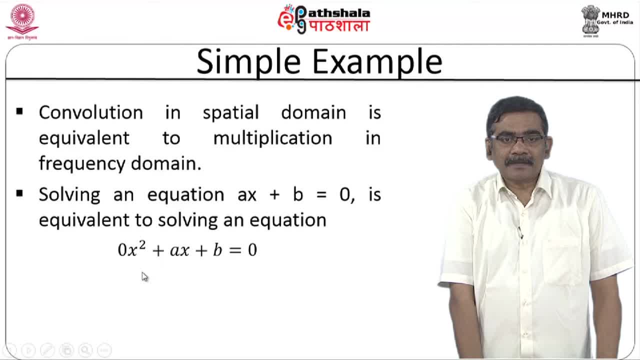 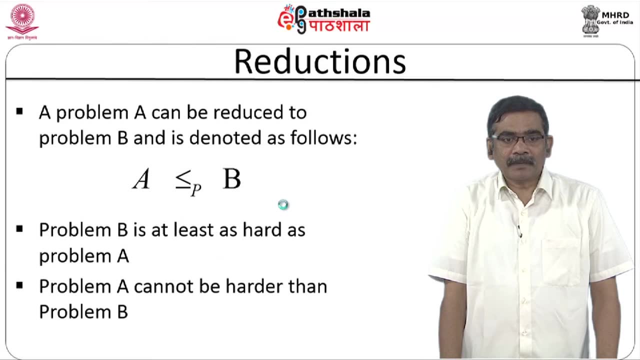 to another problem like this, That is, 0 into X square plus A, X plus B. we can solve that and that constitute the solution of the original instance. In other words, we can reduce a problem A to problem B and this can be represented like: 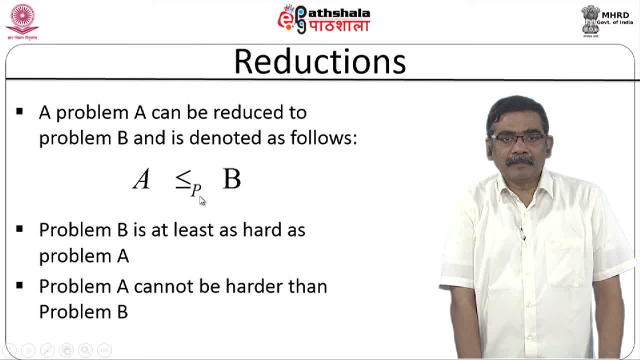 this, where this P is nothing but polynomial P. So the logic is: the problem A is reducible to problem B. What does it indicate? It indicates two things. One is: problem B is at least as hard as problem A and problem. 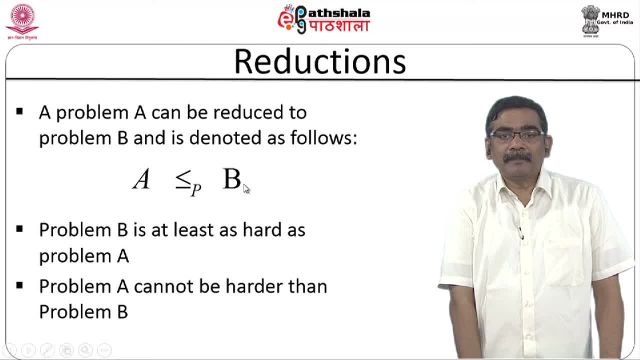 A cannot be harder than the problem B. In other words, the logic is very simple. I am given a problem, and if I could able to reduce that to another problem which is easily solvable, then I can come to a conclusion that the given problem is also a simple problem. 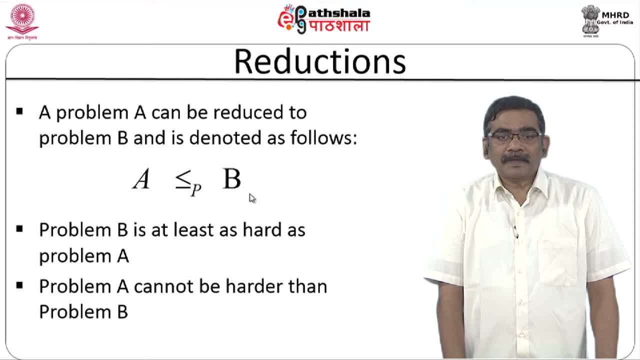 On the other hand, if my problem is reducible to another problem which is very difficult to solve, then my problem is also becoming very, very hard. So you can see the underlining point. that is, we will use this reduction to indicate the hardness of the given problem. 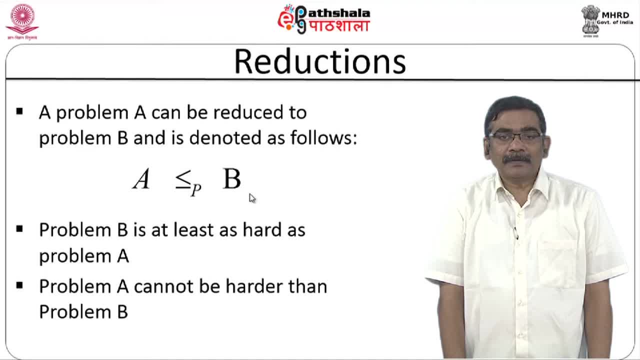 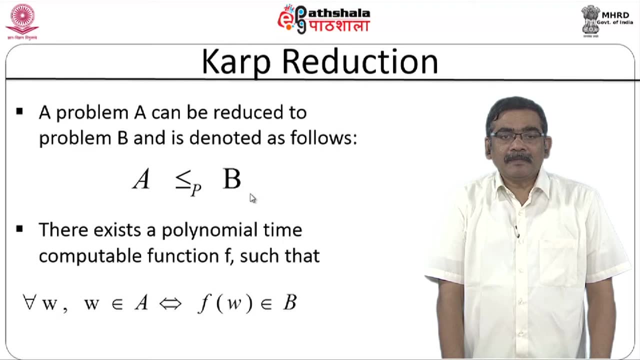 In other words, what we are going to do is we are going to use this reduction as an important tool for giving a proof of the algorithm. hardness Carp reduction is different from the Turing reduction, So here the logic is very simple. The problem A can be reduced to p. 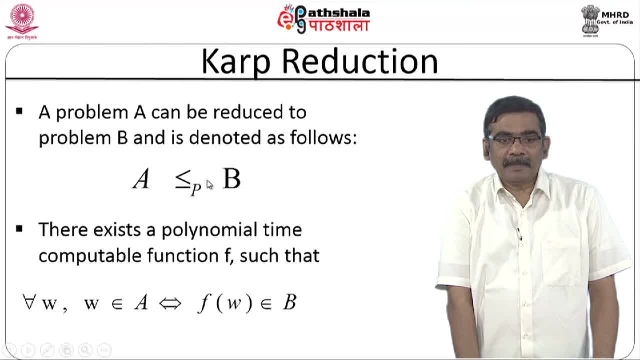 Problem B in polynomial time p can be represented like this, provided if there is a polynomial computation function, f, such that if there is an instance w and if this instance is the instance of the problem A, then f of w should belong to the problem B. 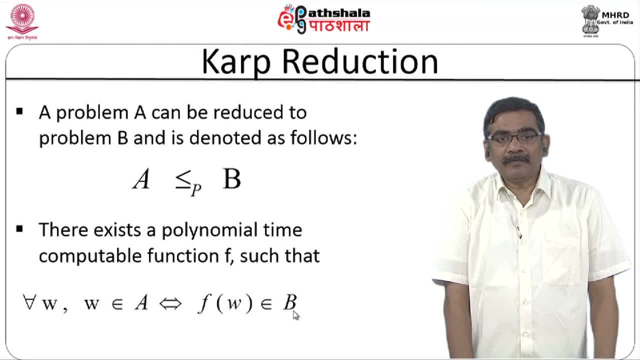 That means what we are going to do is we are going to transform the instance of problem A to another instance of problem B and we are going to solve that using the solver of the problem B, and we are going to show that, if the s instance 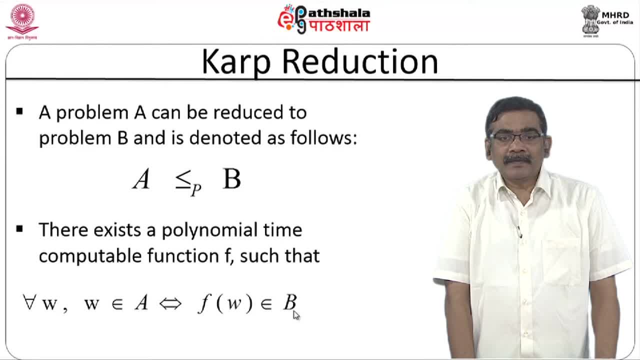 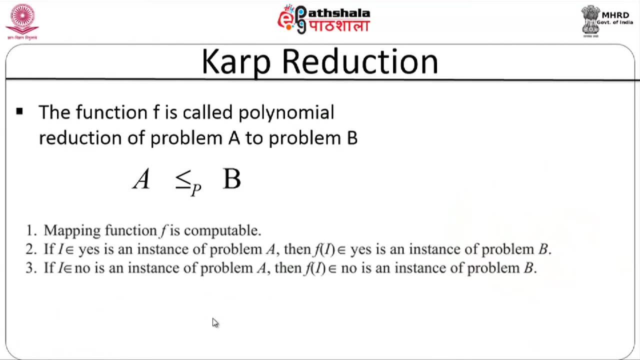 of problem A is equivalent to s instance of problem B, We can say that the solutions are also equivalent. So that is the logic of this particular step. So we can call this in polynomial reduction, So that means we can say that this reduction is carried out in polynomial time. and these 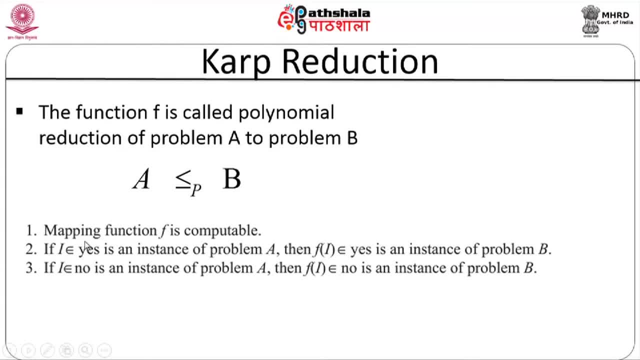 things must be applicable. That means the mapping function f? f should be computable by an algorithm and this function should take care of the instance, such that if i is the instance of the problem I, then f of i is also a s instance of problem. 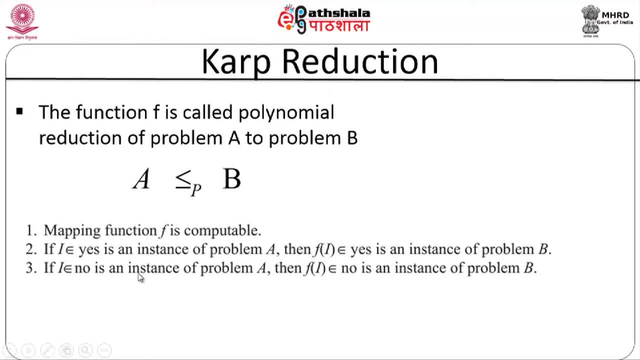 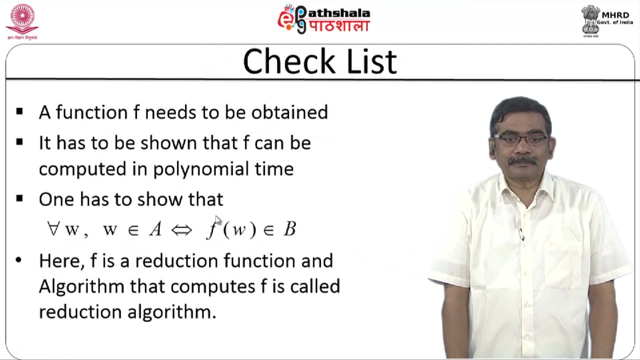 B And similarly, if the instance i is no instance of problem A of i gives no instance, which is also the instance of b. If anyone able to give all the checklist, then we can say that it is a corp reduction. So the checklist for reduction is like this: 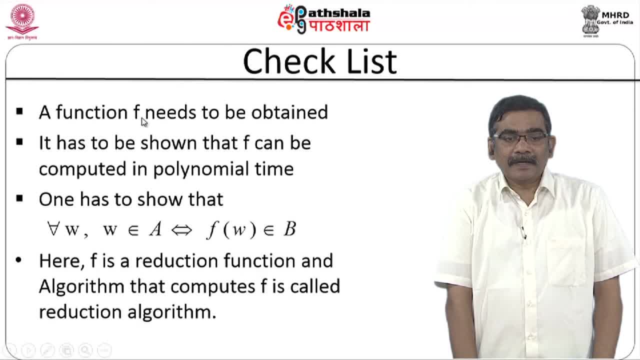 The first task is we have to find a function f that needs to take the instance w and it should provide an output, and we have to show that the output of that is equivalent to the instance input of the original problem. And if anyone could give you a proof that f can. 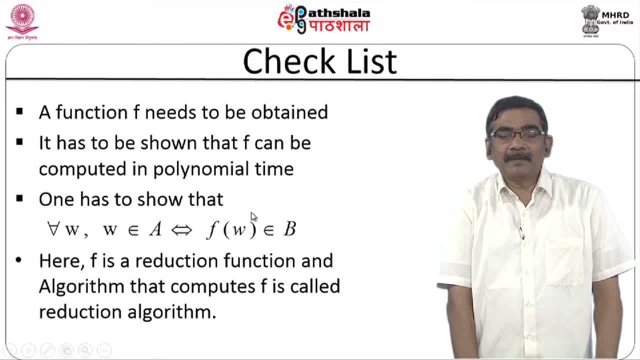 be constructed In a polynomial time, then we can call that as the corp reductions. In this case f is called the reduction function and the algorithm that computes f is called reduction algorithms. So the important aspect of NP complete problem is the obtaining of this reduction function. 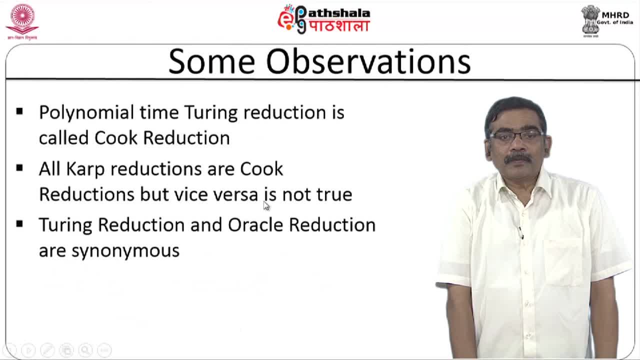 So once we have that, fine, we are ready for giving the proof of NPC. So the polynomial time reduction is also known as Cook reduction. These are some of the important observation that have been made out. That is, the Turing reduction if it can be done in a polynomial. 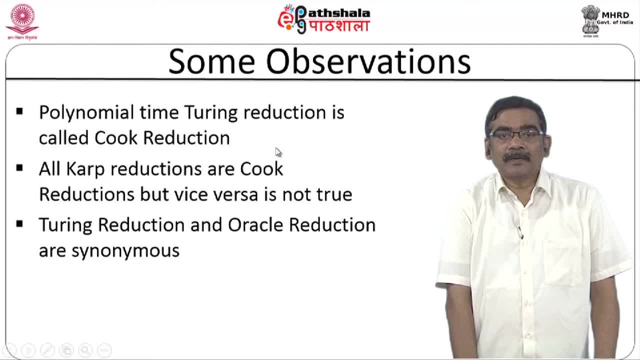 time. I have already mentioned that it is Cook reductions And Turing reduction is also known as the Oracle reductions. So that means we can say that the transform and conquer domain algorithms are mostly coming under this sort of Oracle reduction category. Oracle reduction is same. 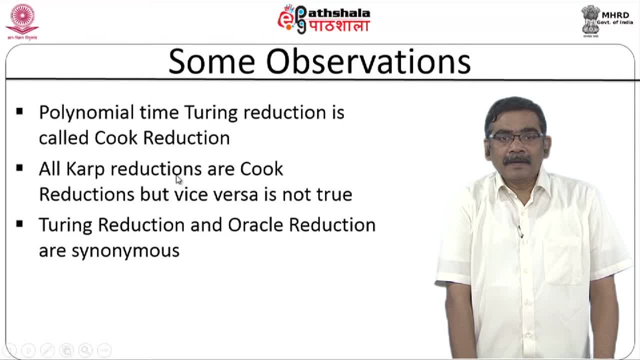 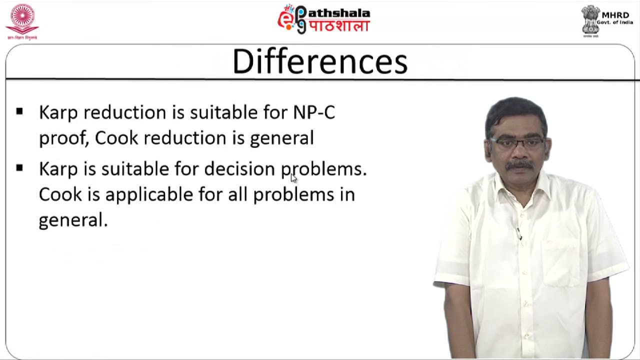 as the Turing reductions. All corp reductions are Cook reductions. So that means Cook reduction is a superset. But the vice versa is not true. That means an Cook reduction need not necessarily be a corp reductions. So that means there is a subtle differences and this slide illustrate. 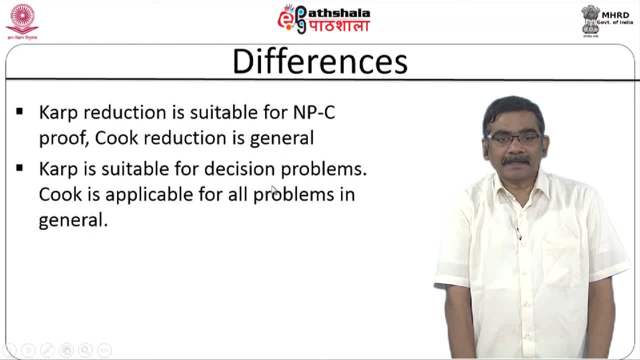 the differences between these two categories. Corp reduction is heavily used for giving the proof of NP complete problems, But whereas the Cook reduction is very general in nature, So for NP complete proof corp reduction is very important. So that means we have to transform the instance of problem A to the 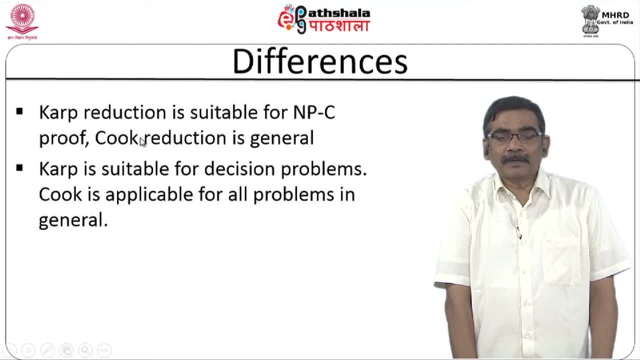 instance of problem B, Then we have to show that the output of that is same as the original instance And corp reduction is very suitable for decision problems. But whereas Cook reduction is applicable for all problems in general, That means it is applicable for the optimization. 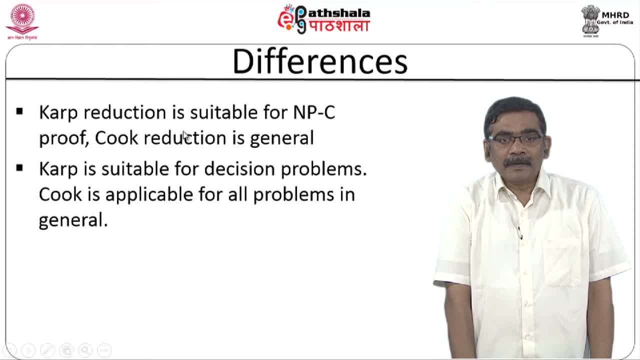 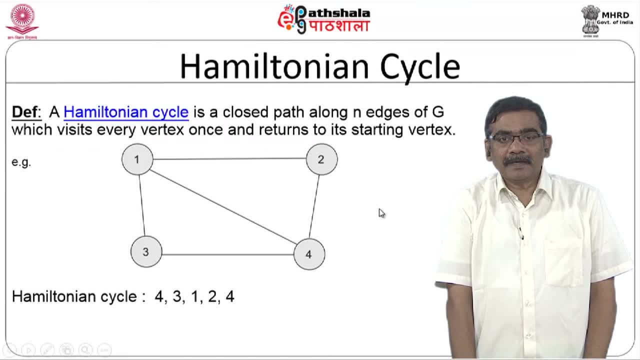 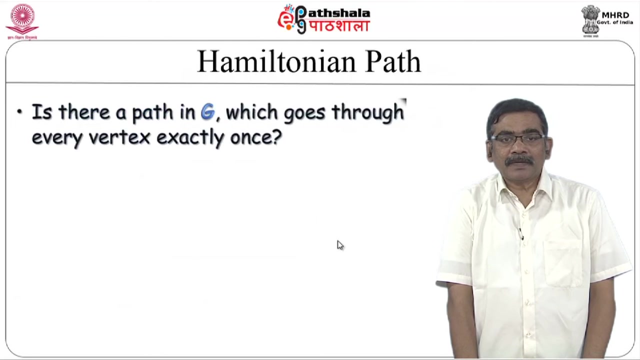 problems also. So I have given a problem and I am asked to convert that to a another problem called Hamiltonian path problem. What is a Hamiltonian path problem? In Hamiltonian path problem also, we are given a graph G. Our objective is to find a path which goes through every. 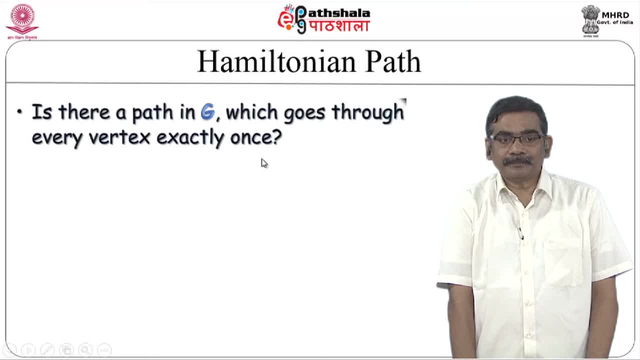 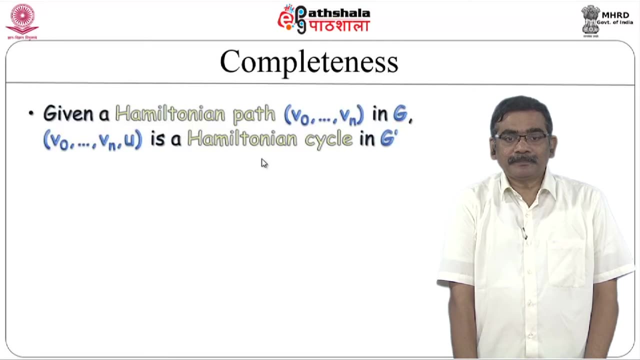 vertex only once It is a path. So the question is How you will convert a cycle to a path or a cycle to a path or path to a cycle. So that means it has to satisfy this criteria of completeness. 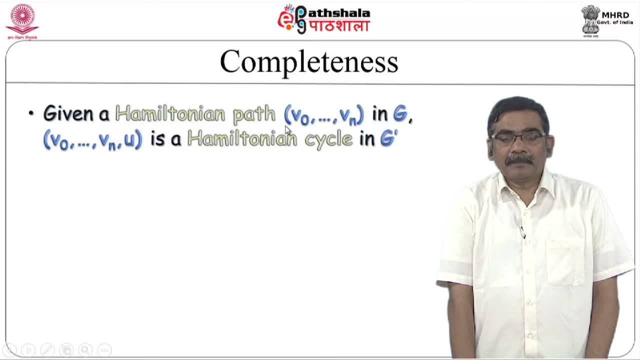 What I can do is I can take a Hamiltonian path, v naught to v, n in G, and I can insert a node U as the adjacent node of all the nodes. If that is the case, then a cycle is created. So that means now you can see that a path 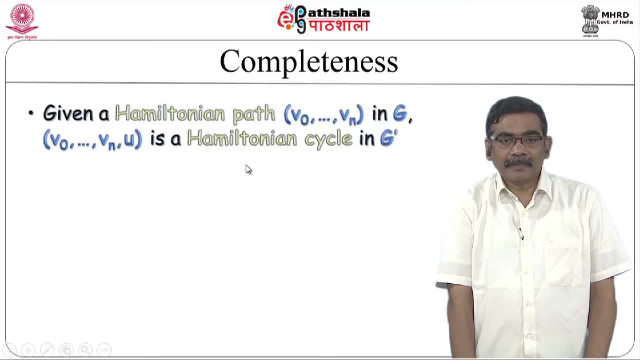 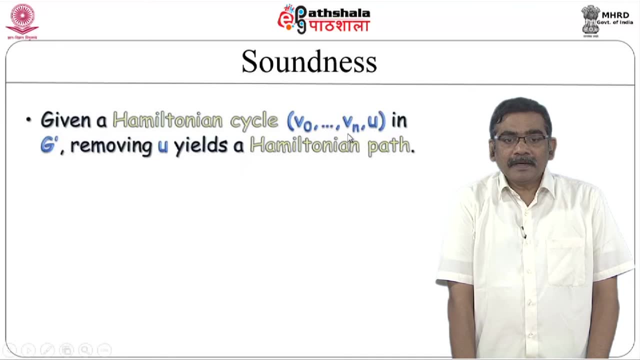 is reduced to a cycle. So this property is called completeness. Suppose, if I remove this node U, automatically the cycle becomes an path. Imagine like this: I have a cycle and if I remove a vertex, then suddenly that cycle becomes a path. In other words, this is called: 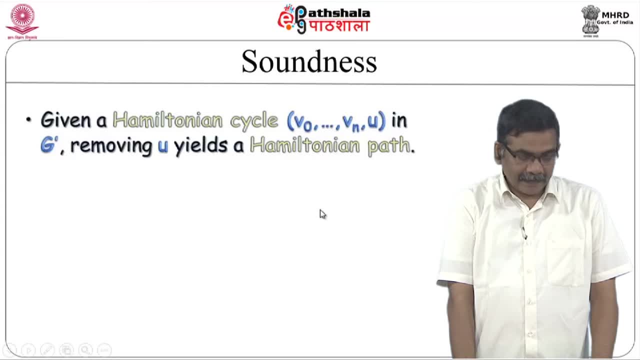 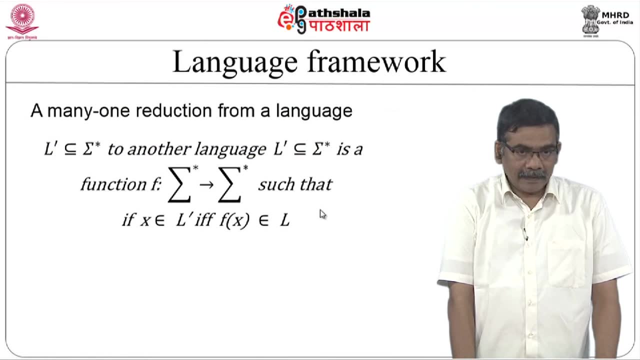 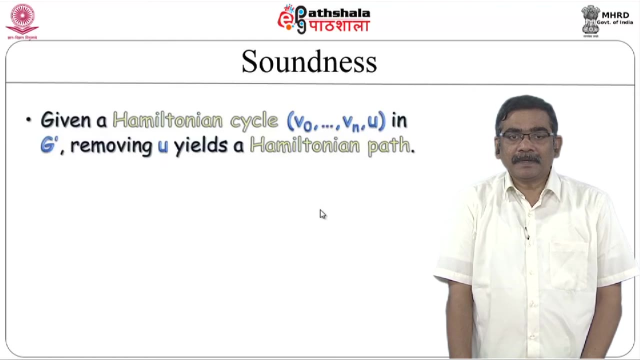 soundness. In other words, I can say that one problem can easily be converted to another problem, and this what we are calling as the reduction property. In other words, this is the kind of what is a reduction we are going to carry out for our NP-complete problems. Now we 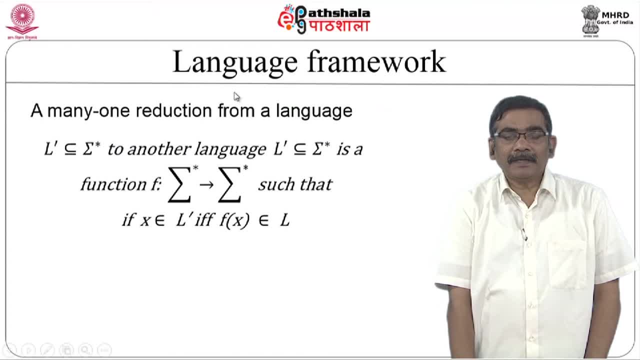 will put everything into a language framework. Please recollect all the terminologies that we discussed, like alphabet string. a set of string is a language. So using that language, we can give you a formal definition of this. So this is the carp reduction. So you have many to one reduction from a language, L prime. 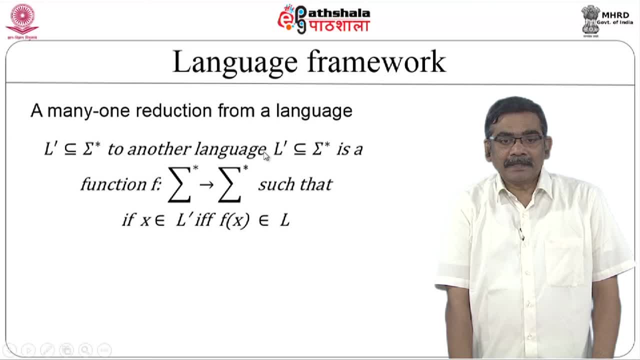 So to another language we can give a set of string. So what kind of a reduction can be done? Here is a new definition of a different type of series, which is called clique reduction to another language. L is a function. as I said earlier, this is going to be a function. f, where 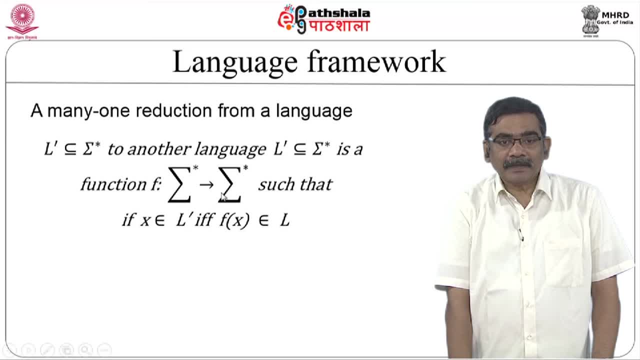 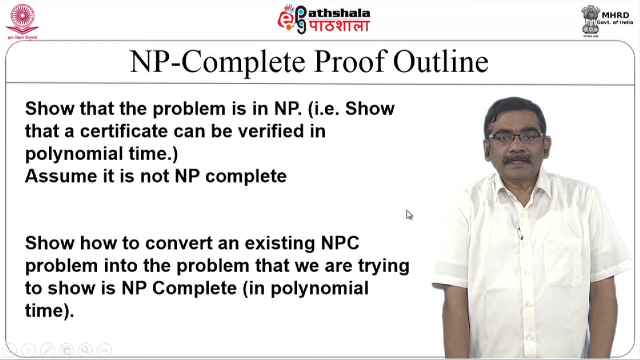 I am going to transform the instance from one thing to another, and if x belongs to the language L prime, then f of x belongs to the language L. This is the formal definition of what you say, the car predictions. So now, using this, we want to create a proof outline. 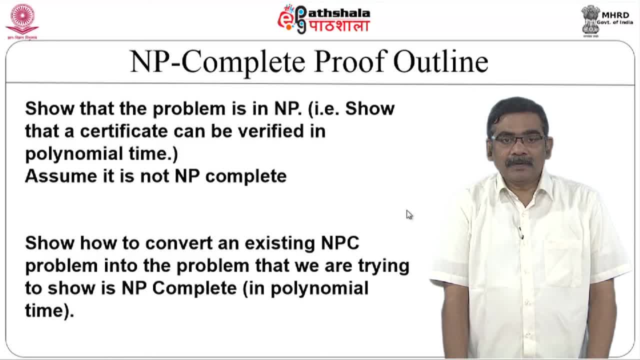 For example, if somebody gives a problem A, they want to know whether the problem is NP complete or not. then what are the steps one needs to follow? The first step is we have to show that the problem is NP. That means we assume that as of now, no easy solutions are available to solve that. 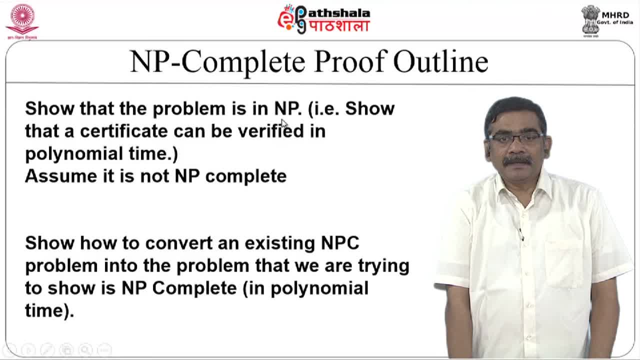 So we say that it is NP problem. Second, there must exist a certificate. so that means the verification should be able to complete in polynomial form. So we have to prove that there exists a certificate and verification algorithm so that the verification can be done in a polynomial time. 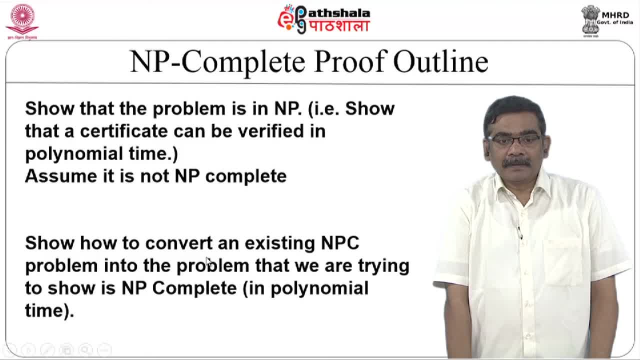 This is the another aspect. Third aspect is now you take a well-known NP complete problem and use car prediction and you try to reduce the problem. So this is the other aspect: If someone could able to do that and if someone prove that it is done in a polynomial time. 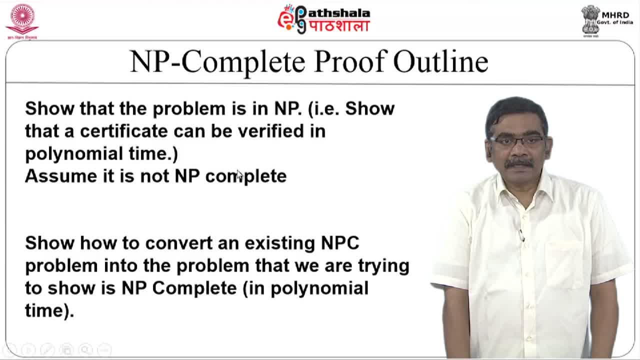 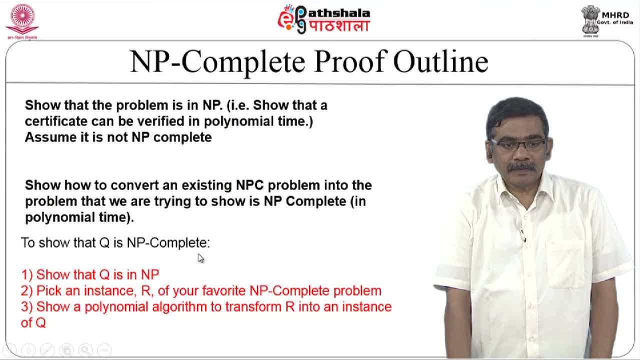 fine, then we can come to a conclusion that the given problem is going to be a NP complete problem. So this is what we are going to do. So we are going to take the problem Q, which is in NP, So we want to prove that this Q is NP complete. 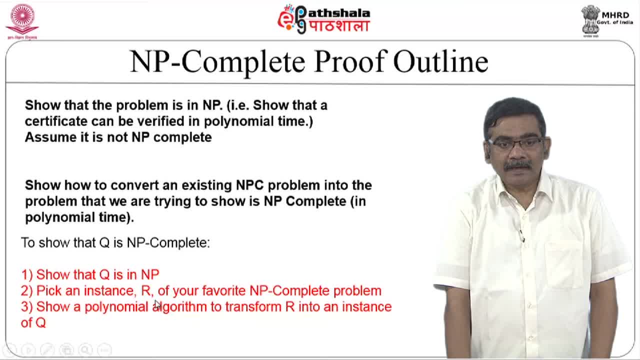 So what we are going to do is we are going to pick an instance R of favorite NP complete problem. As we said earlier, SAT problem form a sound foundation for this. We can take an instance and we have to go for a polynomial reduction algorithm to transform. 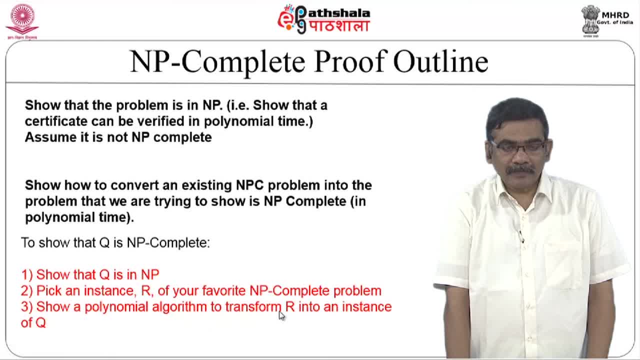 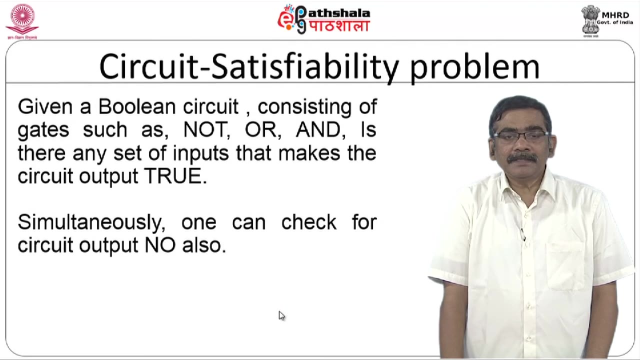 the instance of R to the instance of Q And if someone able to prove that the reduction is possible, then we can argue that Q is as odd as NP. complete problem, therefore, it is a difficult problem to solve. This is the kind of proof we are looking for. 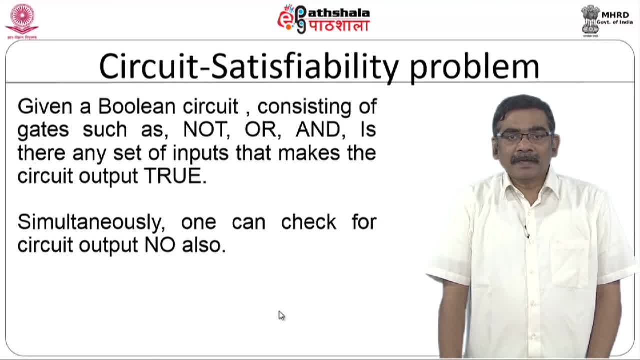 So that means, In other words, I am given a problem that I need to show that it is NP complete. So what I will try to do is I will take another problem. then that problem is NP complete. So I will try to reduce that to this problem so that I can say that my given problem is. 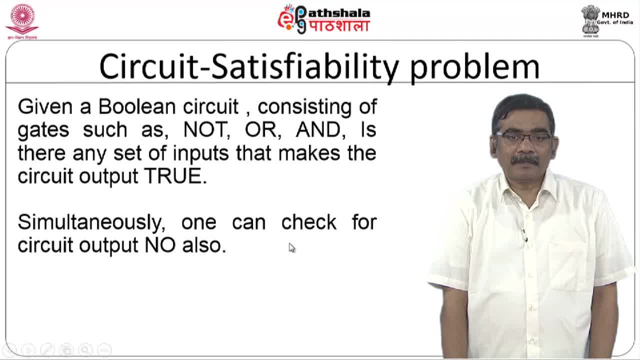 as good as what is NP complete. So that means, in other words, I am given a problem that I need to show that it is NP complete. So I am going to say the hard problem, which is well known. Now let us apply this framework for the set of problems. 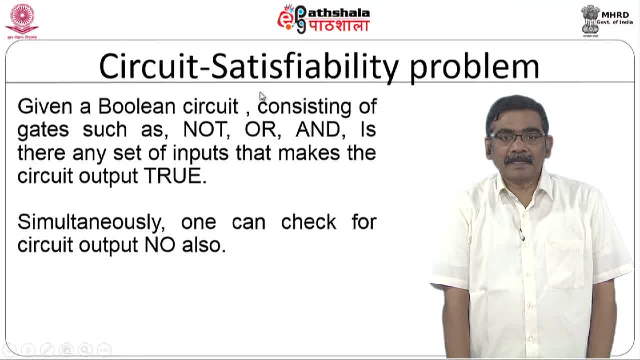 For this I am going to take the circuit satisfiability problem. So circuit satisfiability we have seen in the last module we are given a Boolean circuit. So Boolean circuit consists of lots of gates like NOT OR and AND. as I said earlier, the logic is very simple. 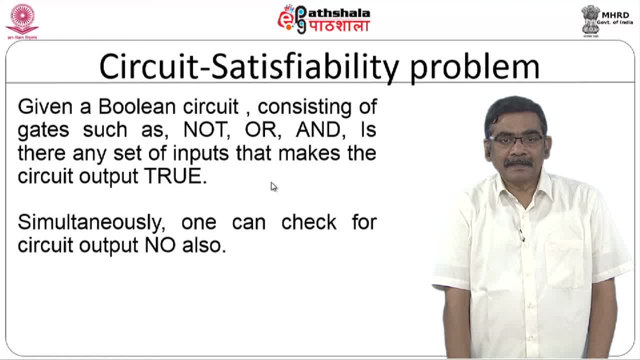 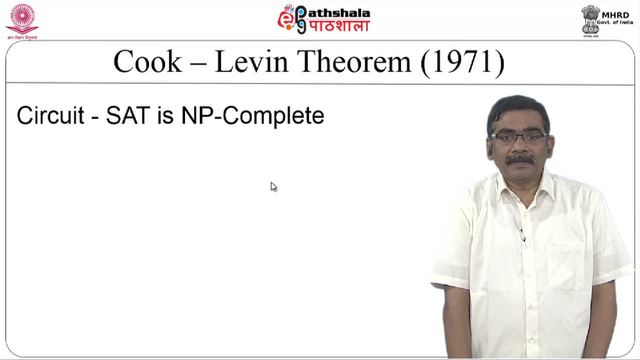 We have to give an assignment that make the circuit output as true. Simultaneously one can check the circuit output for NO also. This is a important theorem. So Cook Levin theorem, proven independently in the year 1971, states that circuit SAT is NP complete. 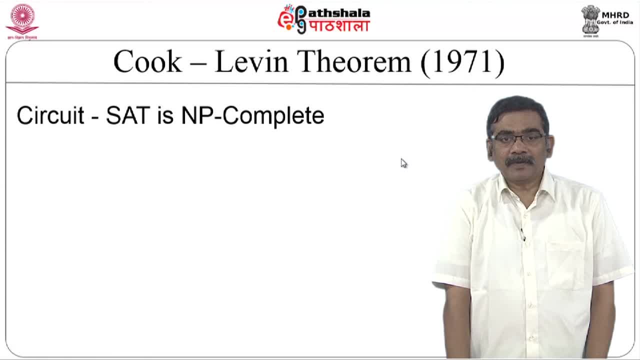 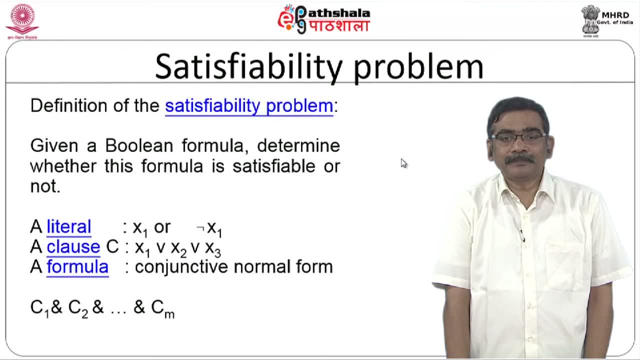 As I said earlier in the last module, if the number of inputs becomes large, then finding the solution becomes very, very difficult. Now we will take one relative problem: satisfiability. this also we discussed in the last module. This is formula or expression, SAT. we are given a Boolean formula.